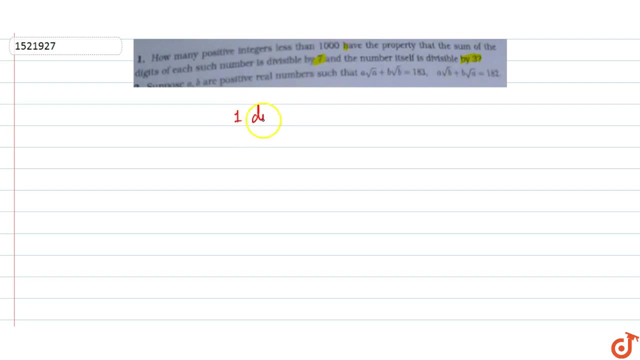 So what can be the number? It can be a one-digit number or a two-digit number, or a three-digit number. It can be a three-digit number. So what will be the one-digit number? It will be of type A, 12-digit number: A and 3-digit number. 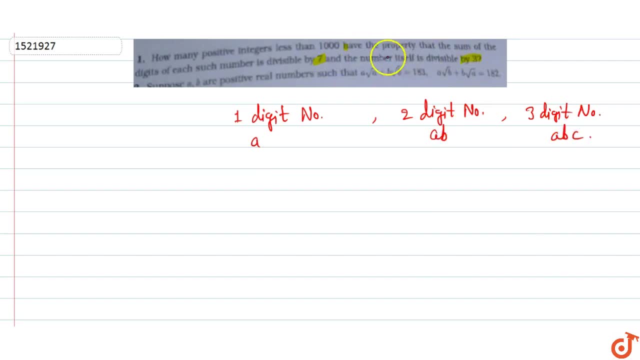 It will be of type A, 12-digit number A and 3-digit number C. Now that number has the property that the sum of the digits of each, such that the number is divided by 7.. The number is divisible by 7.. 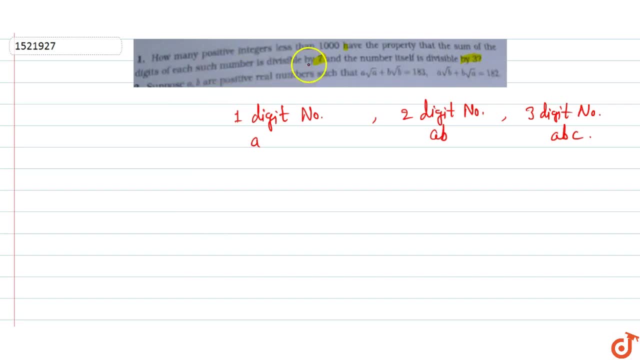 Means the sum of the digits of each number is divided by 7.. So what should be its sum? It should be divided by 7 and the number itself should be divided by 3.. The number should be divisible by 3.. 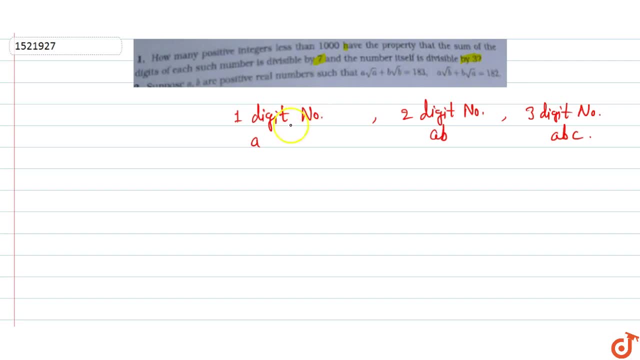 Means the sum of the digits is divided by 3.. So can it be a one-digit number? It can't be. The sum of the digits of each number is divisible by 7, and the number itself is divided by 3.. 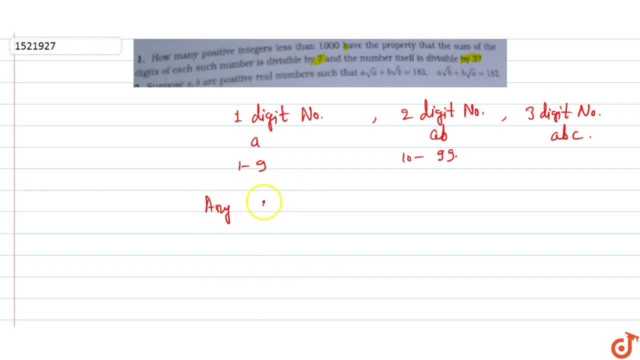 So any number whose sum of digits is divisible by 7.. The sum of the digits is divisible by 7. So it must be a divisible number, Because its sum of digits is divisible by 3. It has to be divisible by 3.. 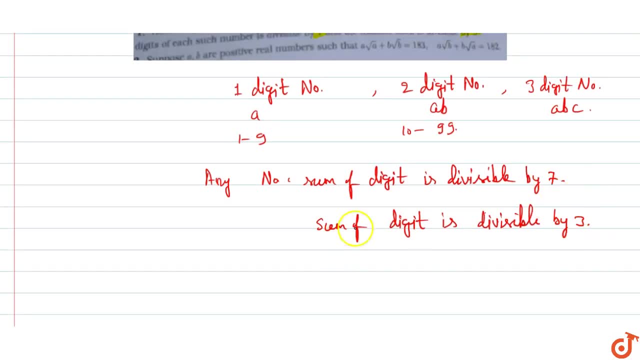 It means the sum of the number is divided by 3.. Then the number should be divided by 7 and the number does not have any divisive sense, but the sum of the digits of the number. it is divided by 3. Then the number should be divided by 3.. 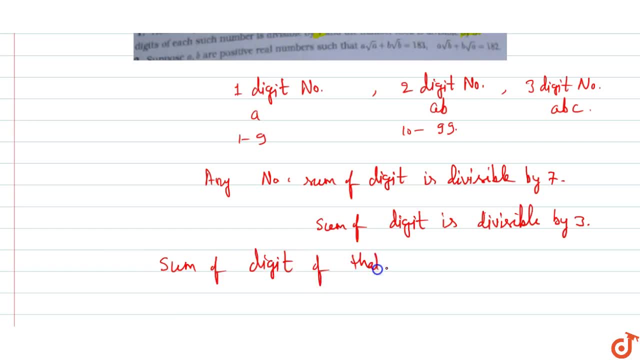 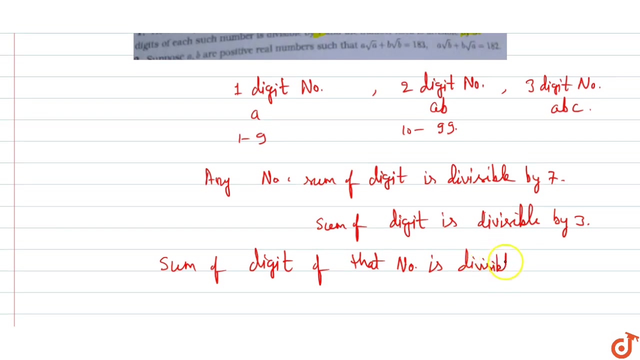 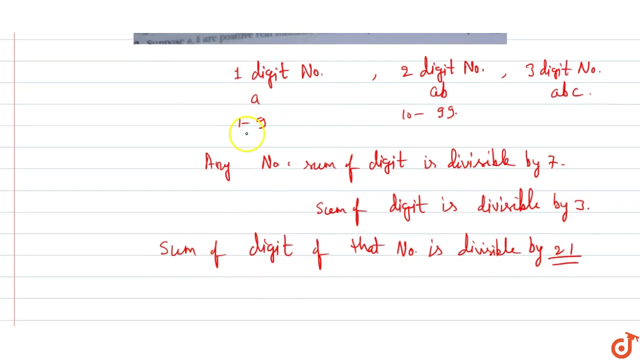 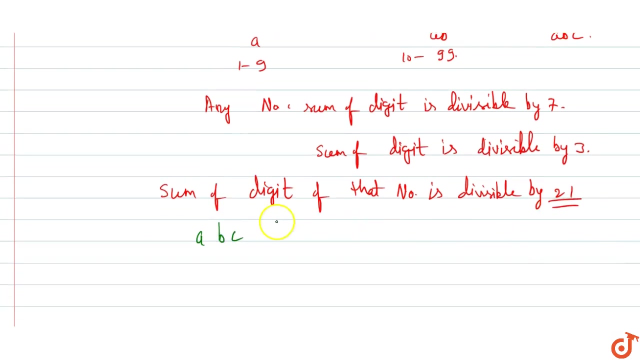 ologia is divisible by 3.. of that number, of that number is so it's divisible by 21. 21 say, divisible only three digits of digit is divisible by 21.. so means sum of digits means a plus b plus c is 21, and type: 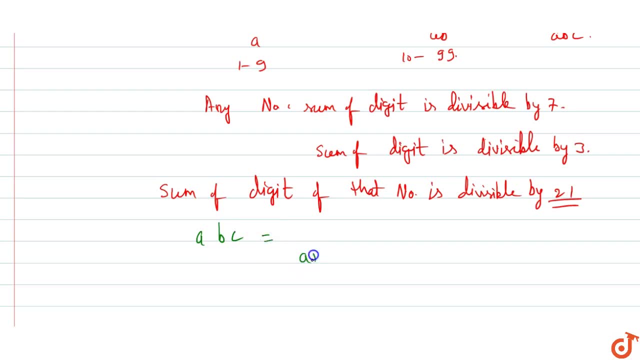 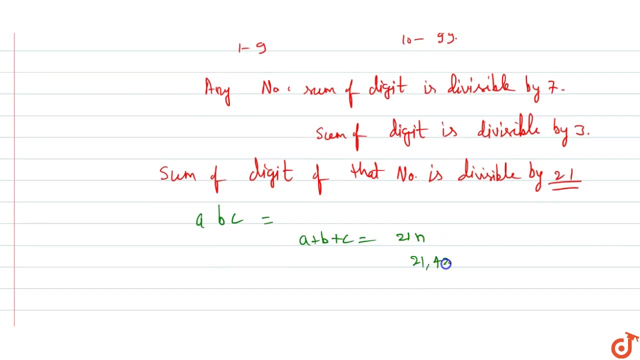 currency means 21, 42, 63. now we got three digits of maximum, something else, okay. nine, nine, nine minutes, nine into three is twenty seven of them, maximum twenty seven. of those may key number is possible only twenty one. so means a plus b plus c is 21. okay now. 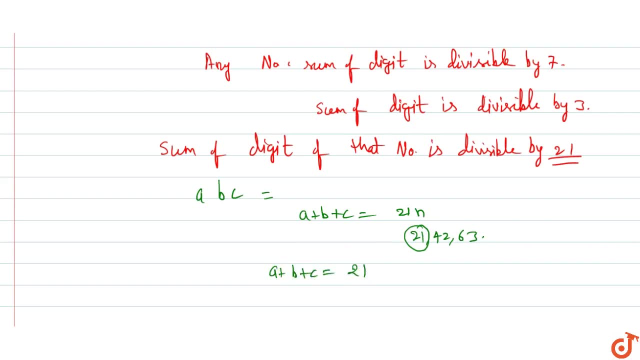 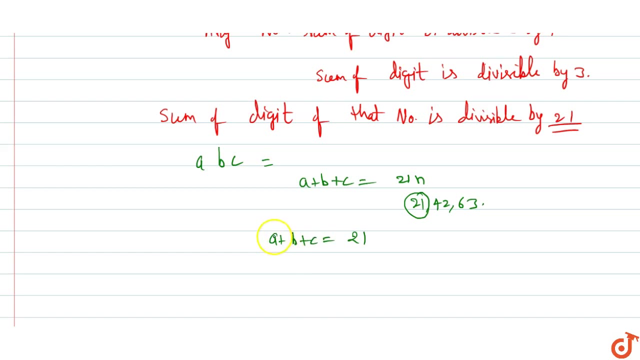 we know that two guys maximum something nine, nine, eighteen. so a key, a key value gives us the minimum three. that means all three numbers are always greater than equals to three. hundred in this case may make necessary condition, however, this is always greater than equal to three. the number of ways when a plus b plus c is equal to 21 and a equal to a is greater than equal to. 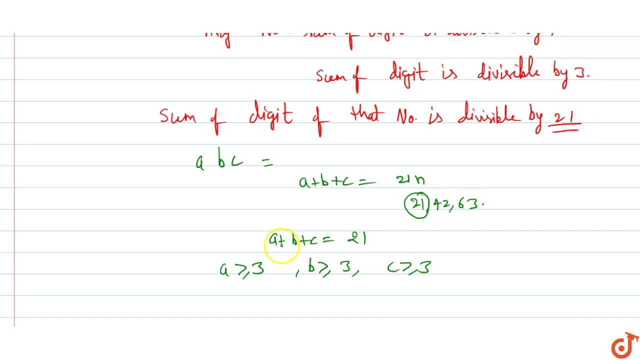 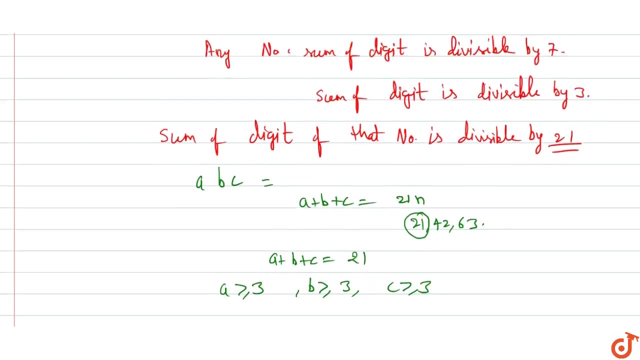 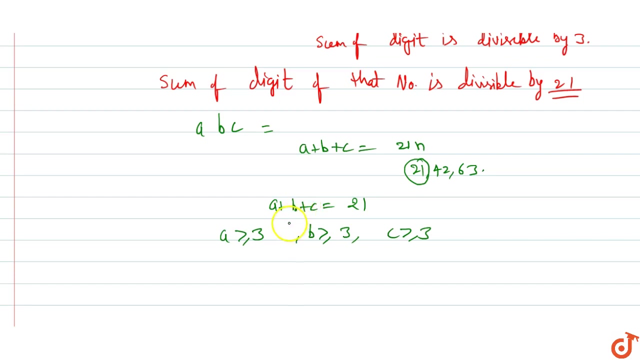 three, b is greater than equal to three and c is equal to equal to greater than equal to three. the number of ways of distributing this: 21 things in three persons when each gets at least three things. three things, okay, so a column can list there three plus alpha will be sucked in where alpha is greater than equal to zero. 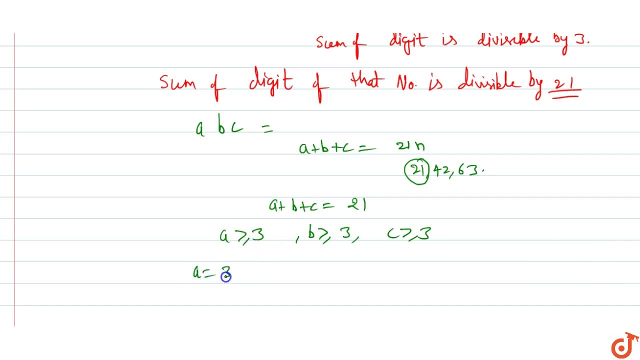 or become carry something: three plus beta, where beta is greater than equal to zero, and c commonly have been three plus gamma, where gamma is greater than equal to zero. so here's a key value: getting three plus alpha, b is three plus beta. plus c is three plus gamma. 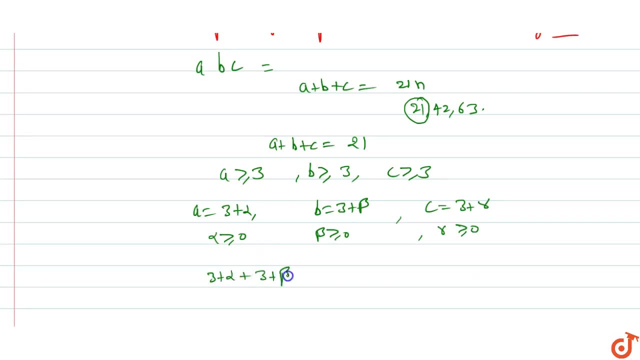 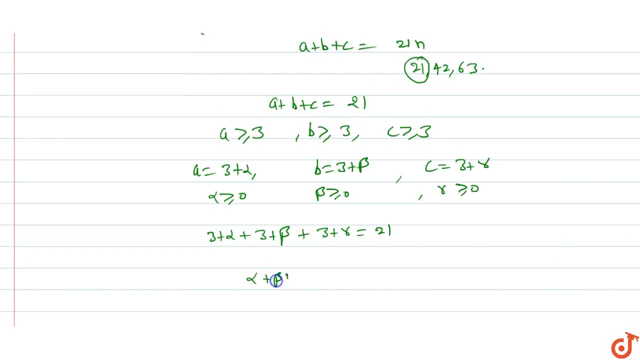 equals to 21.. the value of alpha plus beta plus gamma equals to 21 minus 9, which is equal to 12.. it is equal to 12.. okay, the number of ways of distributing these are 12 things in three persons. with at least each one get any number of things. 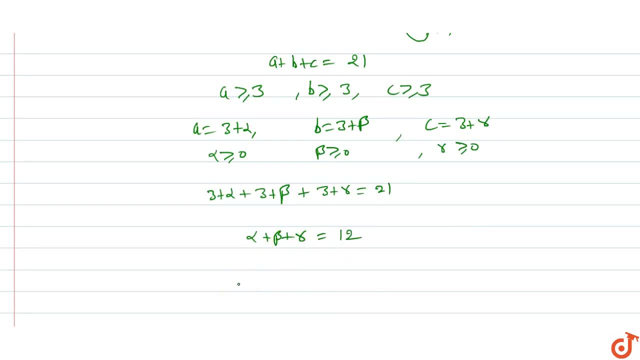 the number of phase counting. this could be again 12 plus three minus one, c three minus one. okay, and different things so are different. yeah, justified. and plus r minus one, c r minus one. so this is equal to 14 c two or fourteen c two could get the 14 into 13 by two, two, six, seven times. 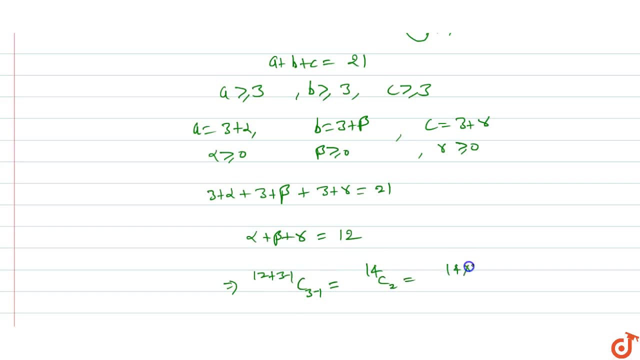 going to fit 11, nine one. the number of ways is 1800. total: 91 numbers: минsch. that number is divided in seven by 14. adjust your kind. there are numbers instead of the end in the end, because the end of the number is not the same. one means lung food식. 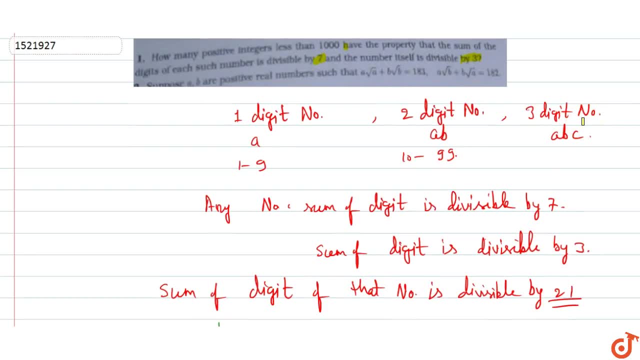 seven and number itself is divisible by three to get a number from a total 91. so this is the answer for this question. 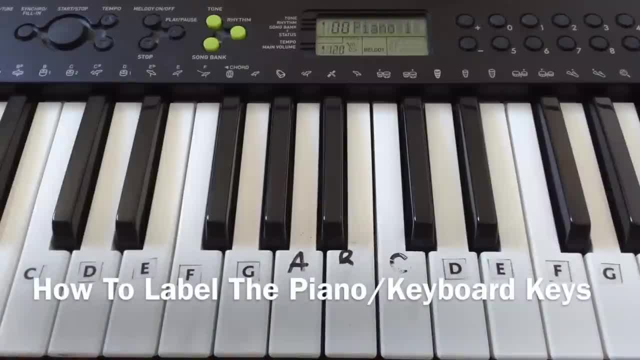 Hi everyone. in this video I'll be showing you how to label the keys on your keyboard or piano. So, as you can see up here on mine it's already actually got the notes, but if yours does not have that, then this video is for you. Ok, so some of the basics, it goes. 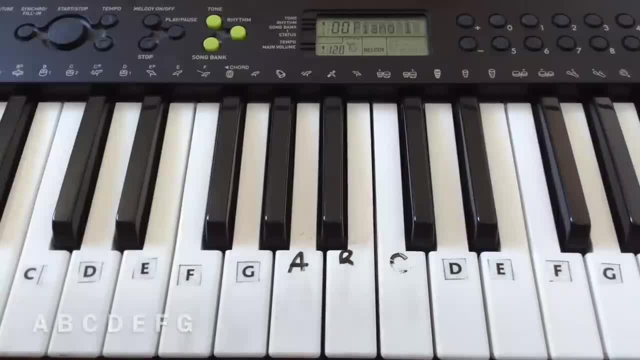 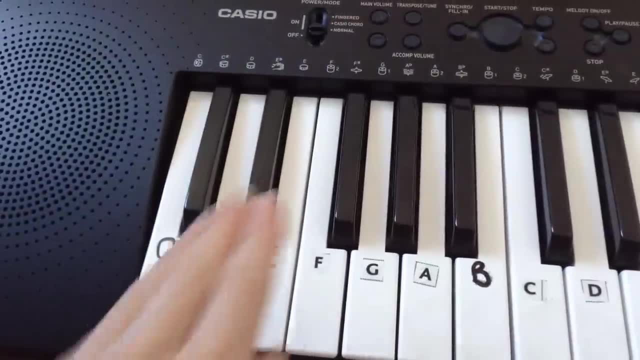 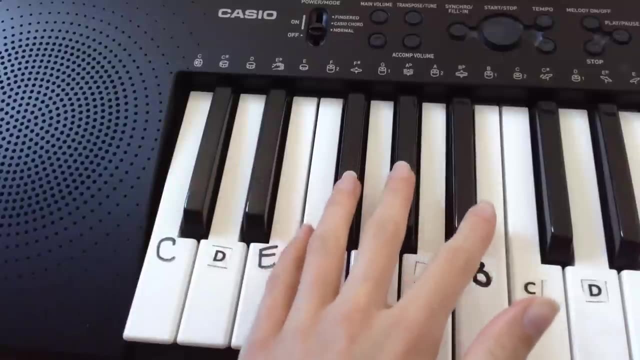 A, B, C, D, E, F, G, no matter what. and it continues, but as you can see on mine, it does not start at A. So what we need to do is we need to find the first three black notes. So mine are here, yours might be here. As you can see, these are in a group, whereas these 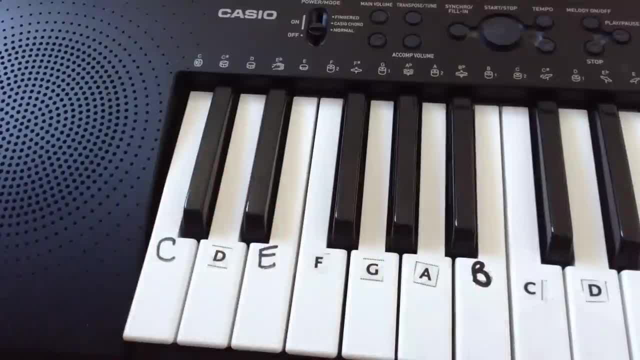 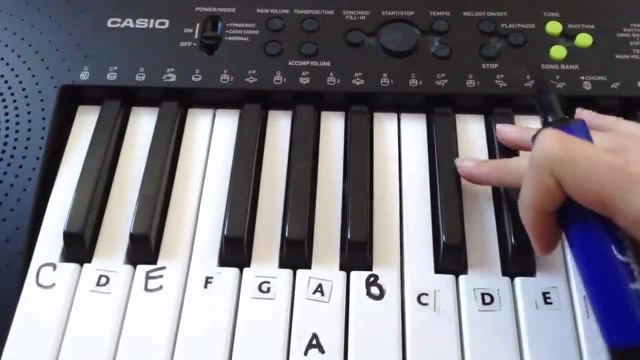 are kind of more separate. I hope you understand what I mean. Ok, so with these three black notes we're going to look at the second and the third, and between those two is an A. So label that A Now to find out where a D is, go onto the first two black notes and then 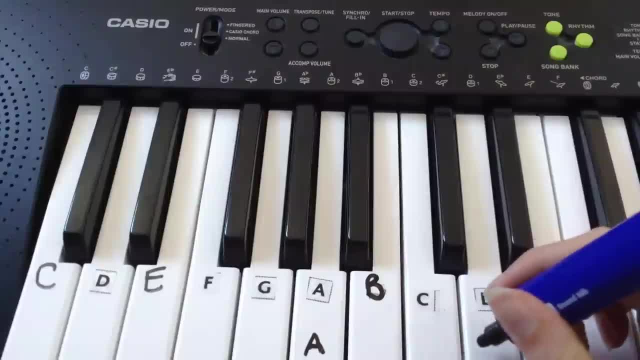 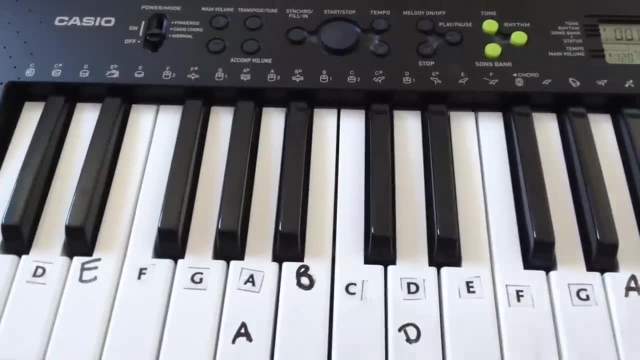 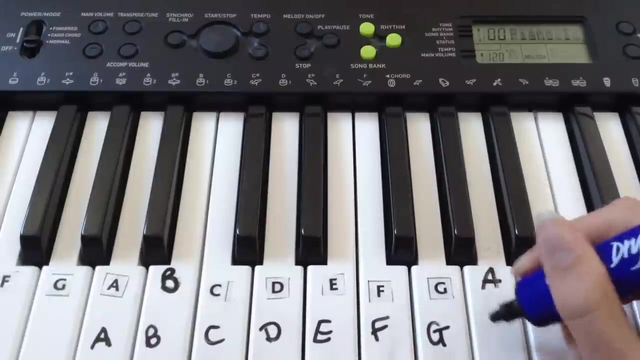 look in between there and write D. Ok, so now we know where A and D are, we can continue writing that all the way down. So A, B, C, D, E, F, and then it would go G, and then, as you might have guessed, we continue with that all the way down. So A, B, C, D, E, F, G. 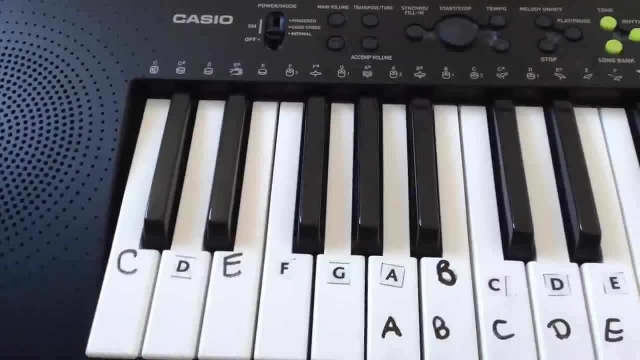 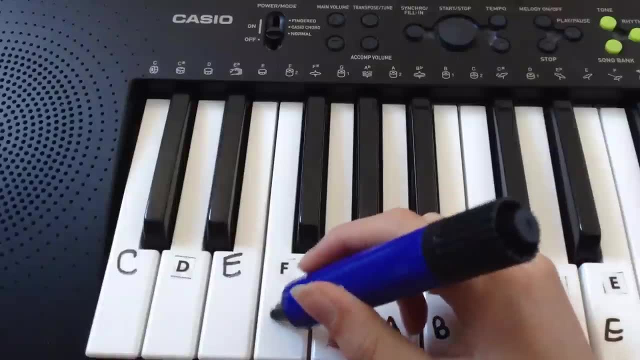 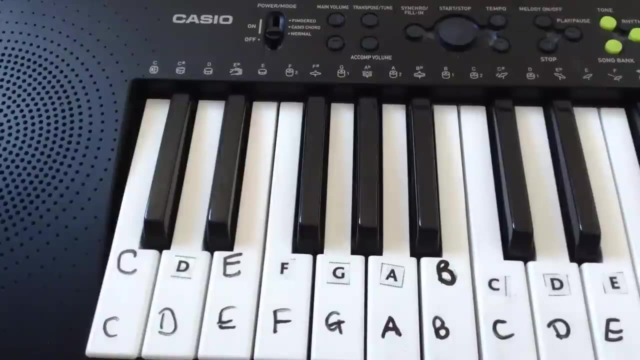 as I said before For the ones before where you first started, we just work backwards. so this is A, so that means it will go G, F, E, D, C. Ok, so that is simply how to label the notes on your keyboard.